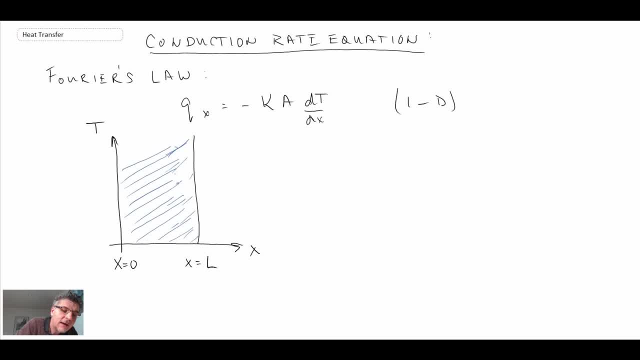 distance along the horizontal. And if we could measure the temperature. let's say we measure t1 here and then, a little further into the solid, we measure t2 and what we find is for one-dimensional conduction. oops, I didn't do a very good job of that. this should be a linear line, a straight line. 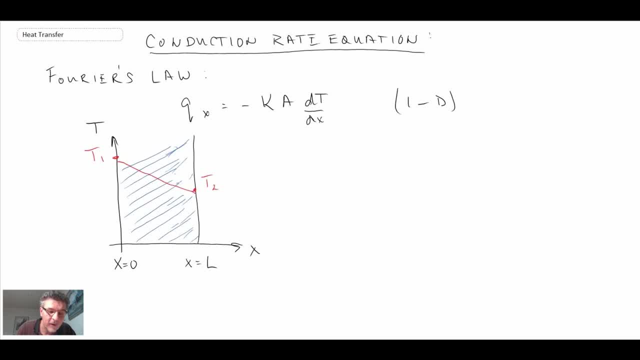 So there we go. that's a straight line connecting x equals 0 to x equals L, t1 to t2.. And then, remember, the heat is going to flow from the hotter to the cooler and consequently, the heat transfer is going in this direction here, and we will take 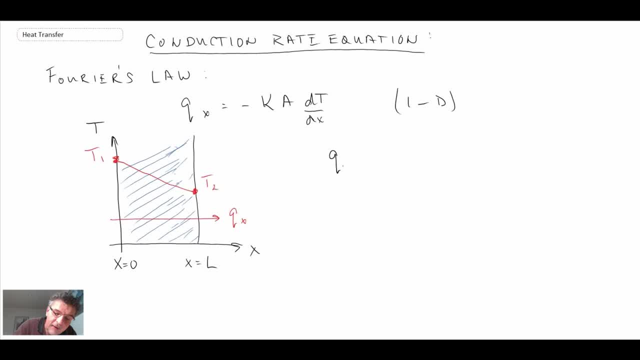 a look at the different terms in Fourier's law. We have qx. that's referred to as being the heat transfer rate, and that can be in watts or joules per second. We already talked about that in an earlier segment. The next term that we have is K. K is the thermal conductivity of the solid that we 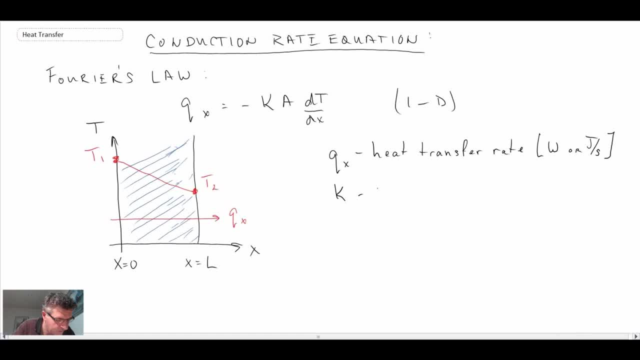 have, or the material that we have the heat transfer going through, And the units of K are going to be watts per meter degrees C, or it could be watts per meter kelvin, And the next term that we have is the cross-sectional area through which the 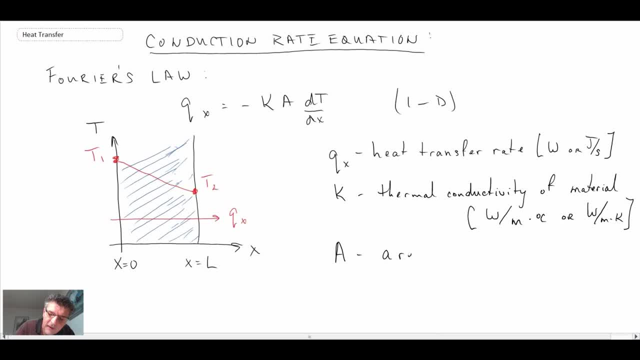 heat is being transferred through. So that's the area of the surface And that will be in units of meters squared. And then, finally, we have dd by dx, that is the temperature gradient in the direction of heat transfer And that is what is driving the heat transfer to take place, And the units there are degrees C per.